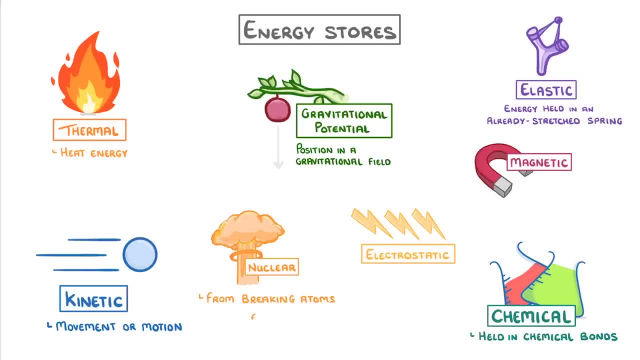 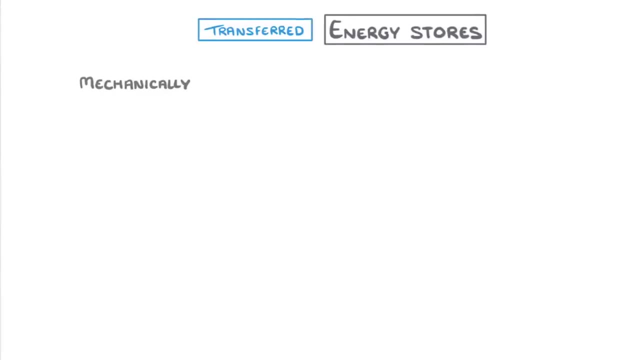 And finally, nuclear energy, Which is what we get from breaking atoms apart. Now, the key idea is that the energy in each of these stores isn't fixed. Instead, it can be transferred from one to another. This could be done mechanically, such as physically stretching an elastic band electrically. 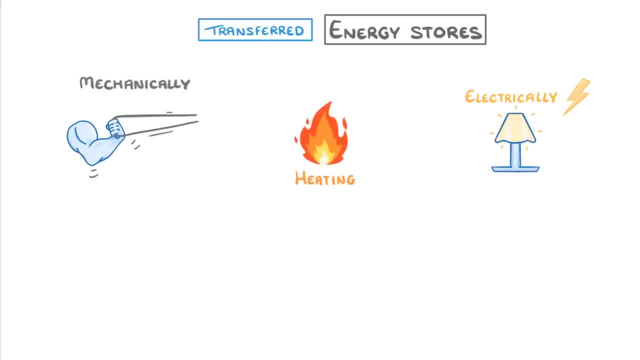 such as plugging something into a socket by heating or by radiation like light or sound waves. When we consider a particular object or group of objects, we can call the collection of matter a system, which is just the fancy term that you need to use in physics. 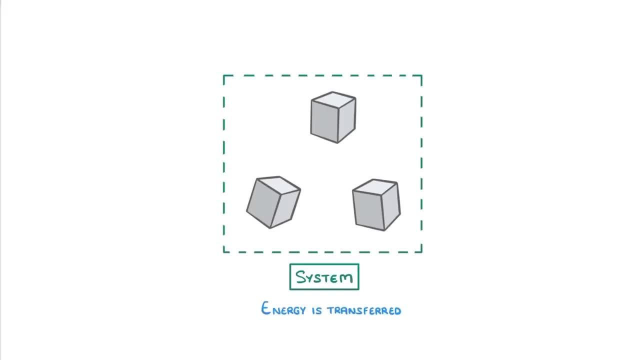 When the system changes, energy is transferred either between objects or between different forms. In an open system, the matter of the system can exchange energy with the so-called outside world, Which is just all of the matter that's outside of our system. 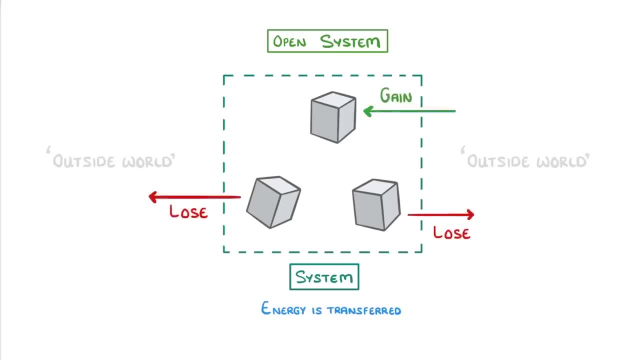 This means that an open system can lose or gain energy as it interacts with the outside world. By comparison, a closed system is separate from the outside world, So neither matter nor energy can enter or leave, And so, even though energy can be transferred within the system, 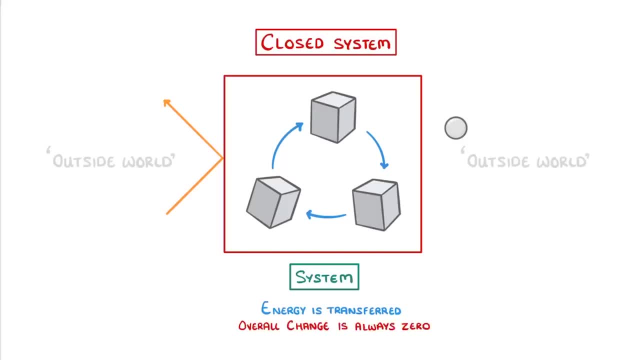 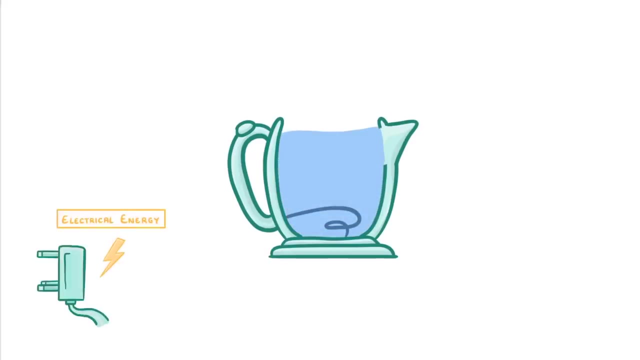 The overall change is always zero. To understand how this actually works in practice, let's take a look at a couple of examples. Imagine we have a kettle and we fill it with water. When we turn it on, electrical energy from the plug socket flows to the heating element of the kettle. 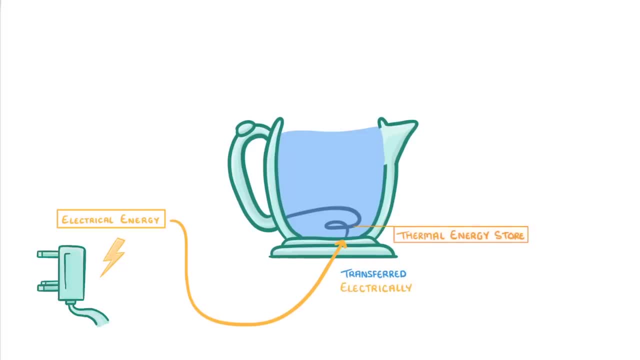 where it's transferred electrically to the thermal energy store of the kettle's heating element, which basically means that the flow of electricity warms the metal heating element. The heating element then in turn transfers the energy over to the water's thermal energy store. 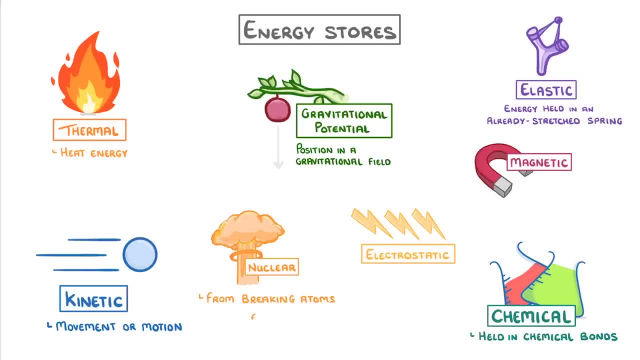 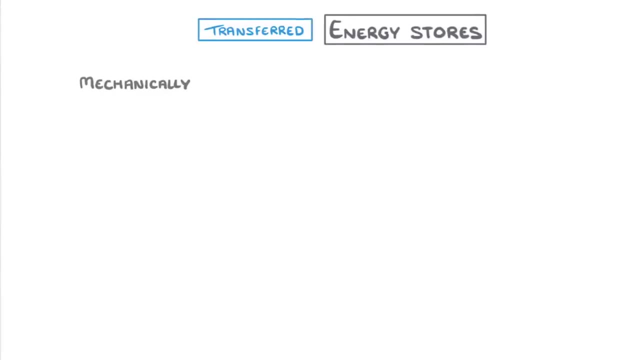 And finally, nuclear energy, Which is what we get from breaking atoms apart. Now, the key idea is that the energy in each of these stores isn't fixed. Instead, it can be transferred from one to another. This could be done mechanically, such as physically stretching an elastic band electrically. 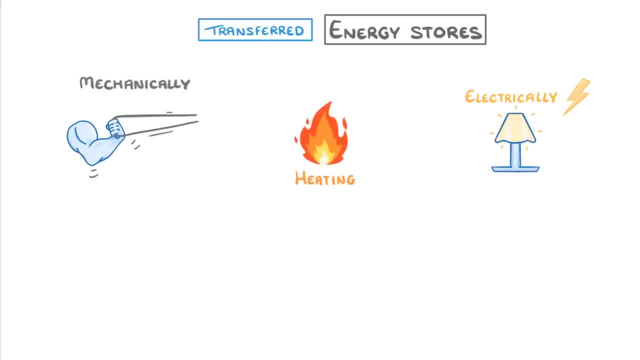 such as plugging something into a socket by heating or by radiation like light or sound waves. When we consider a particular object or group of objects, we can call the collection of matter a system, which is just the fancy term that you need to use in physics. 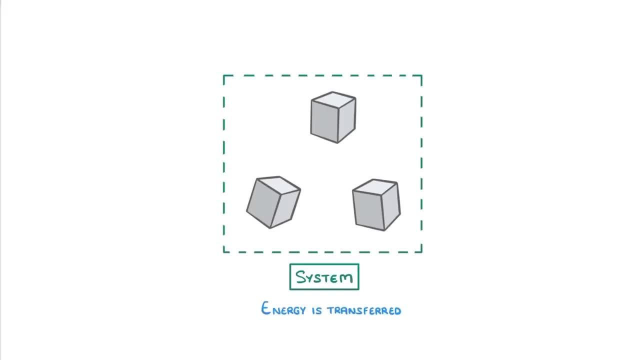 When the system changes, energy is transferred either between objects or between different forms. In an open system, the matter of the system can exchange energy with the so-called outside world, which is just all of the matter that's outside of our system. 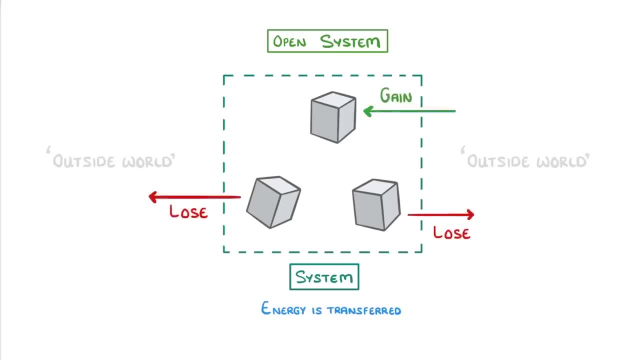 This means that an open system can lose or gain energy as it interacts with the outside world. By comparison, a closed system is separate from the outside world, So neither matter nor energy can enter or leave, And so, even though energy can be transferred within the system, 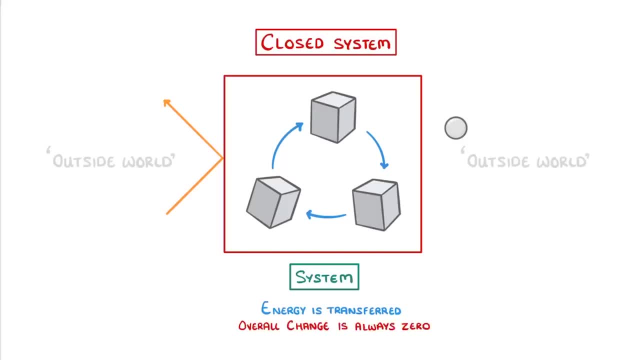 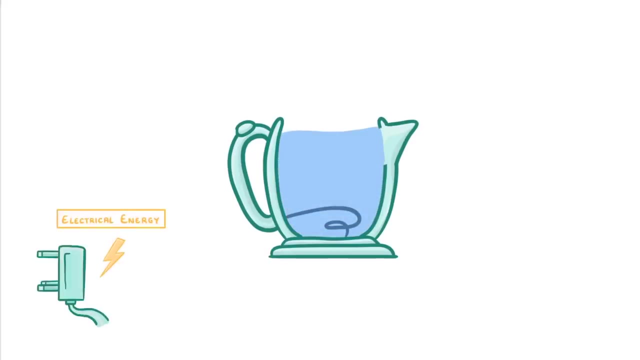 The overall change is always zero. To understand how this actually works in practice, let's take a look at a couple of examples. Imagine we have a kettle and we fill it with water. When we turn it on, electrical energy from the plug socket flows to the heating element of the kettle. 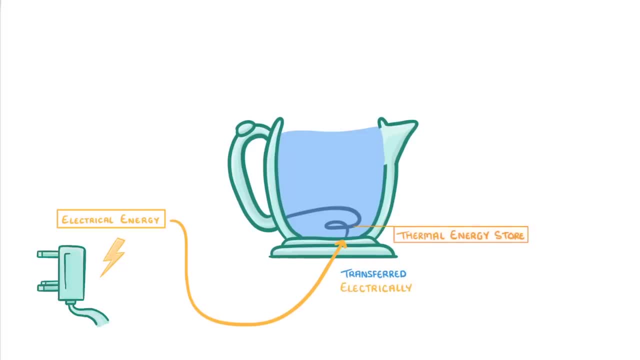 where it's transferred electrically to the thermal energy store of the kettle's heating element, which basically means that the flow of electricity warms the metal heating element. The heating element then in turn transfers the energy over to the water's thermal energy store.